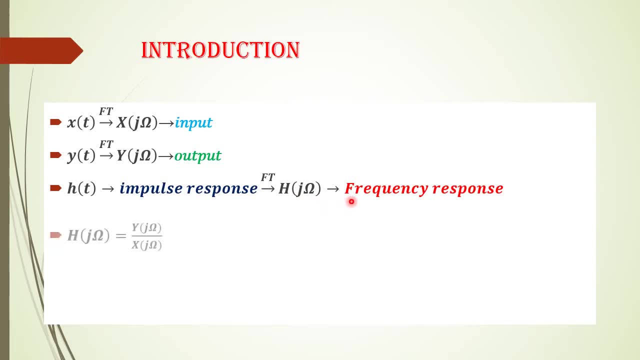 This is also called as frequency response, So it has another one formula. that is output response divided by input response: y of j omega divided by capital X of j omega. Then Fourier transform of d power n divided by d t power n, x of t is j omega power n into capital X of j omega. 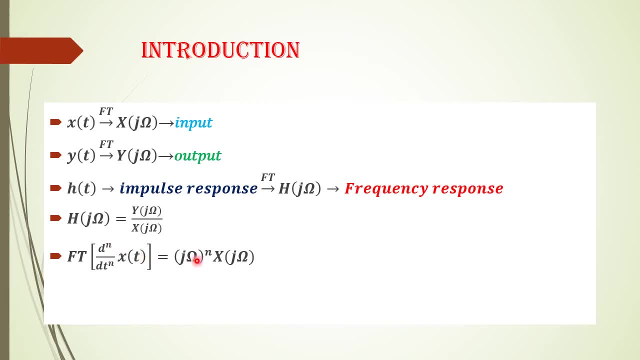 So if the degree n is equal to 2, means then you will be getting j omega, the whole power 2, into capital X of j omega. Then inverse Fourier transform of 1 divided by j omega plus a is equal to e power minus a t into u of t. 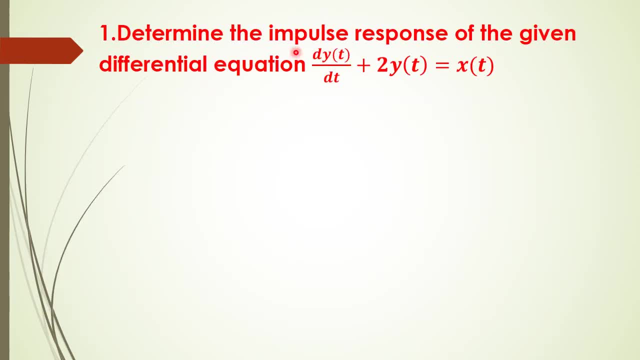 Now let us solve the problem: Determine the impulse response of the given differential equation: d y of t divided by d t plus 2 y of t, equal to x of t. So here in the question they are asked to find the impulse response. 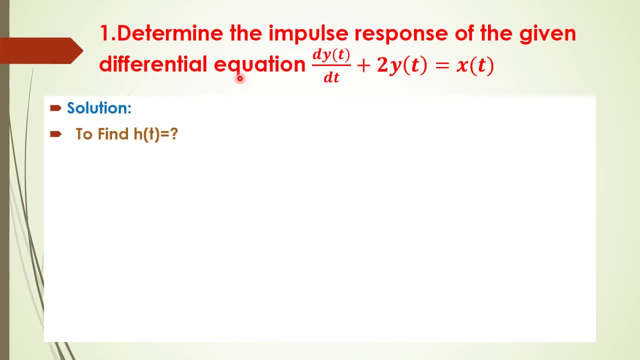 So impulse response means h of t. So we have to calculate what is h of t. So first, d y of t divided by d t plus 2 y of t is equal to x of t. Now we have to take Fourier. 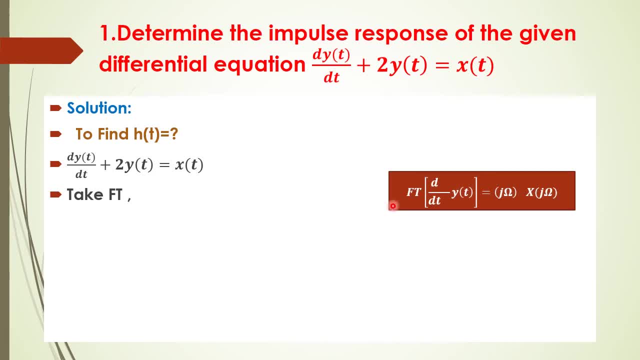 So if we take Fourier transform, Fourier transform of d by d, t of y of t is j omega into capital X of j omega. Already we have seen this. Now you have to substitute it here. So you will be getting j omega into y of j omega, plus 2 into y of t. 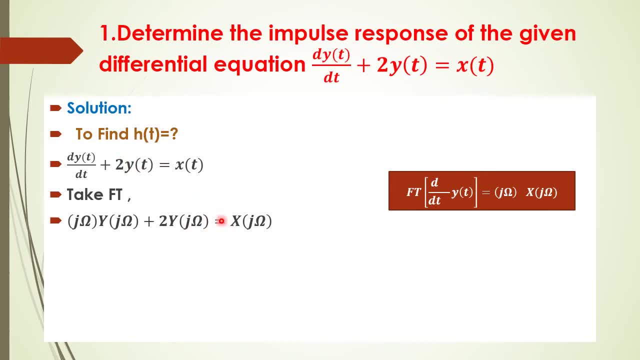 Fourier transform is capital Y of j omega, equal to x of t. Fourier transform is capital X of j omega. Now take y of j omega outside, So you will be getting j omega plus 2. that is equal to capital X of j omega. 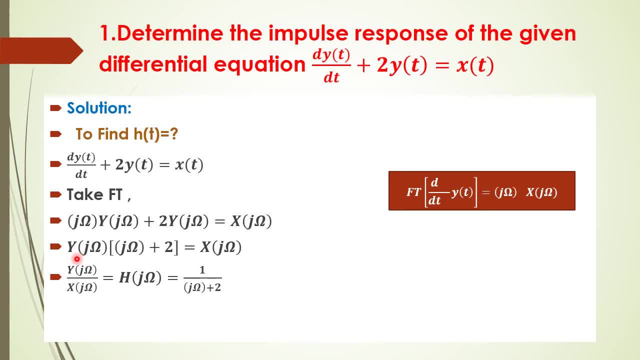 Then you have to bring this x of j omega to the left hand side, So you will be getting y of j omega divided by x of j omega. This is nothing but our frequency response. that is h of j omega. So that is equal to 1 divided by j omega plus 2.. 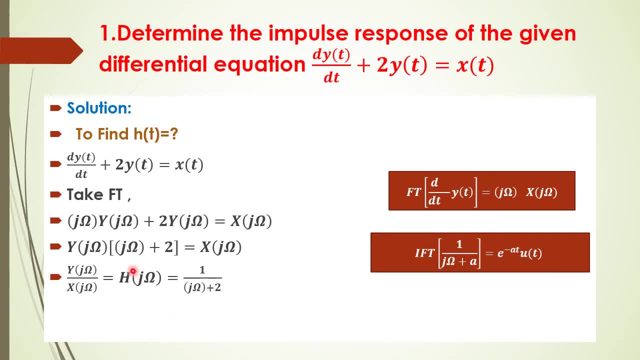 Now we have to find the inverse Fourier transform, Since we need to know what is h of t. So if we know h of j omega means, then automatically, by applying the inverse Fourier transform to h of j omega, you will be getting h of t. 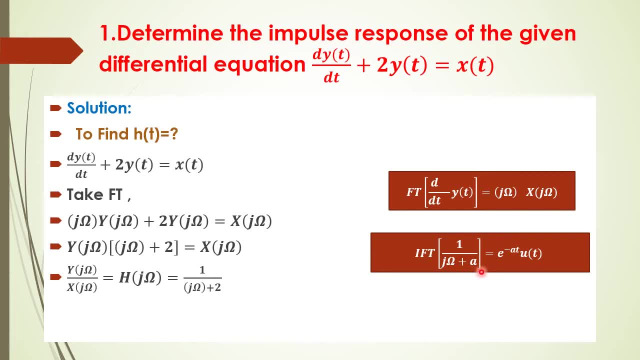 So inverse Fourier transform of 1 divided by j, omega plus a is equal to e power minus a t into u of t. So if you apply this you will be getting h of t equal to e power minus 2 t into u of t. 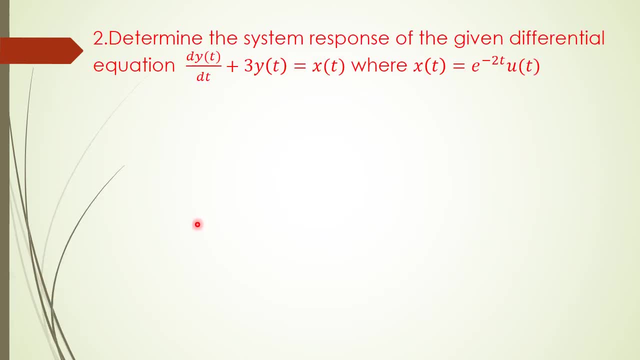 So this is the answer. Then the next problem: determine the system response. So the system response of the given differential equation d? y of t divided by dt plus 3 y of t equal to x of t, Where x of t equal to e power minus 2 t into u of t. 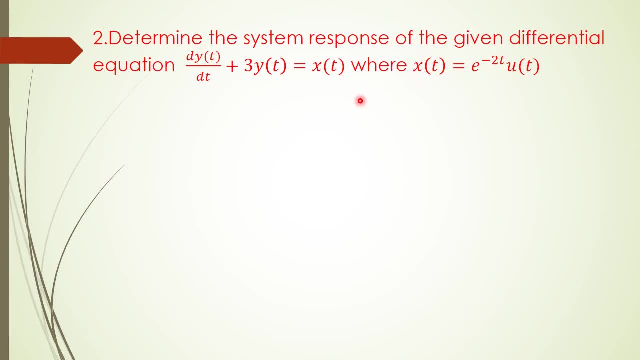 So in this problem the input x of t is also given. Now we have to solve this differential equation and we have to find the system response. So system response means the output response. We have to calculate what is y of t. 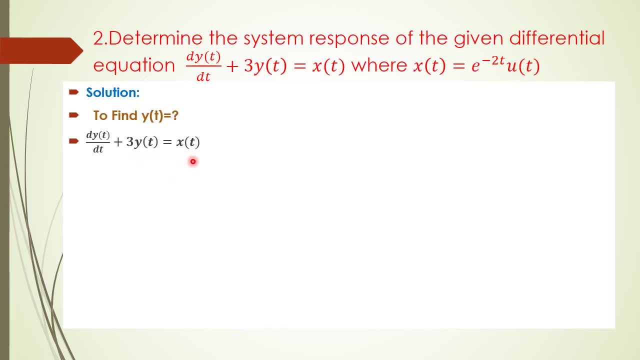 So d y of t divided by dt plus 3 y of t equal to x of t. So d y of t divided by dt plus 3, y of t is equal to x of t. Now take Fourier transform. So by applying the Fourier transform formula you will be getting j omega into y of j omega plus 3 y of j omega, that is equal to capital X of j omega. 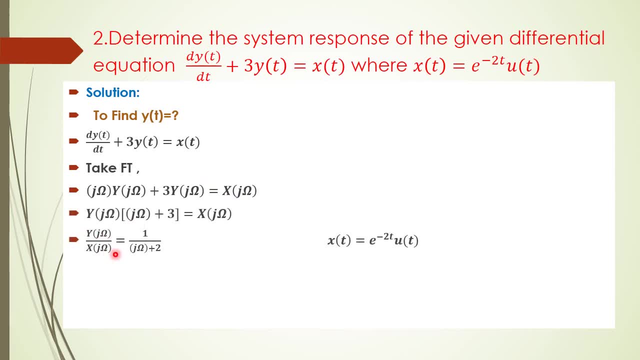 Now on simplifying this, you will be getting y of j omega divided by x of j omega equal to 1 divided by j omega plus 2.. Now in the question it is given x of t equal to e power minus 2 t. 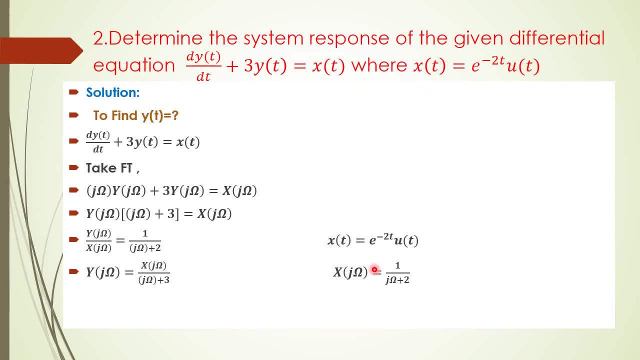 So if we take Fourier transform of x of t, you will be getting x of j omega. So that is equal to 1 divided by j omega plus 2.. Now we can substitute this x of j omega here. So if we substitute x of j omega here, you will be getting y of j omega, equal to 1 divided by j omega plus 3 into j omega plus 2.. 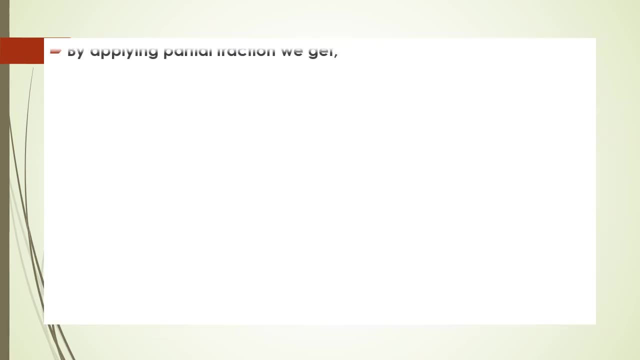 Now we have to apply partial fractions to simplify. So by applying partial fraction we get 1 divided by j omega. So y of j omega plus 3 into j omega plus 2 is equal to a divided by j omega plus 3 plus b divided by j omega plus 2..